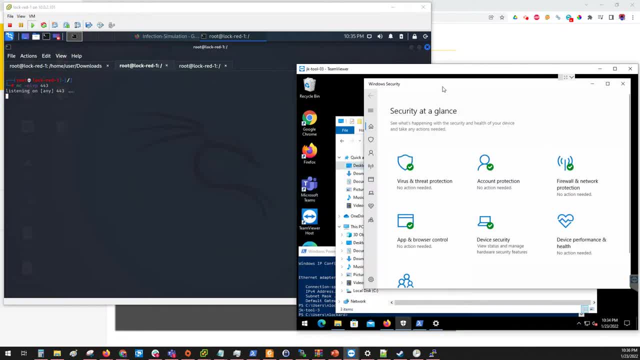 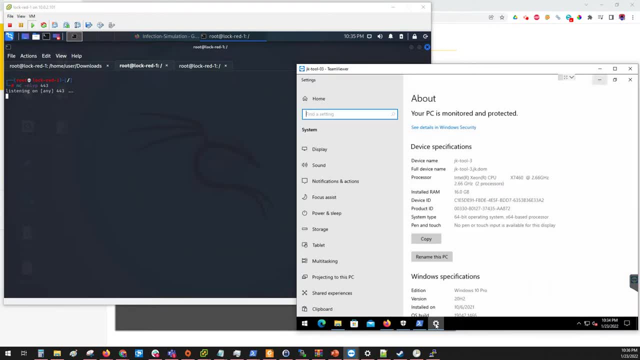 On the right hand side. here is our victim's computer. It is a fully patched and updated Windows 10 system. As you can see, Security Center shows no actions are needed, all green check marks- and this is running Windows 10 Professional 20H2, which is the most updated. 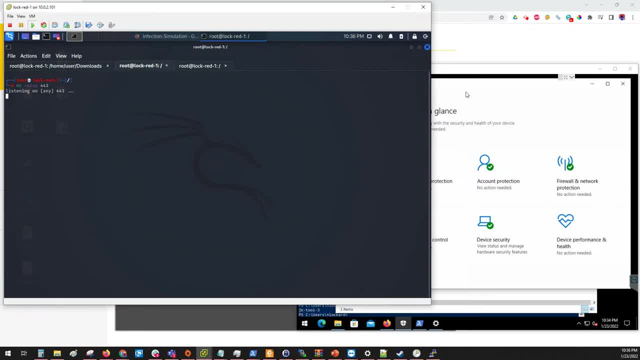 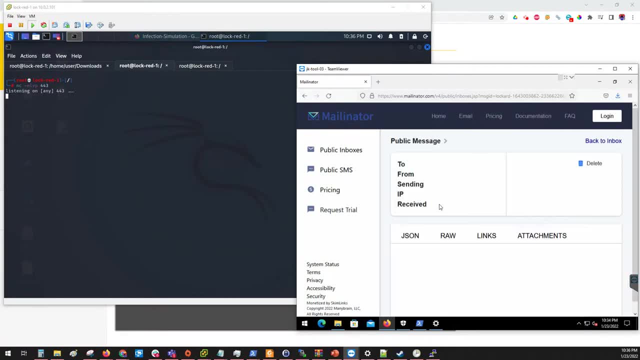 version. The attacker is running Kali Linux, which is here on the left hand side. The hacker's already been configured and is waiting for a connection back. The hacker has sent an email to the victim, as seen here, and the victim is simply going to click and run what is attached. 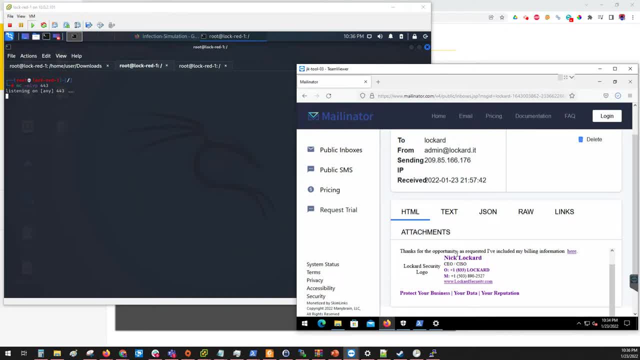 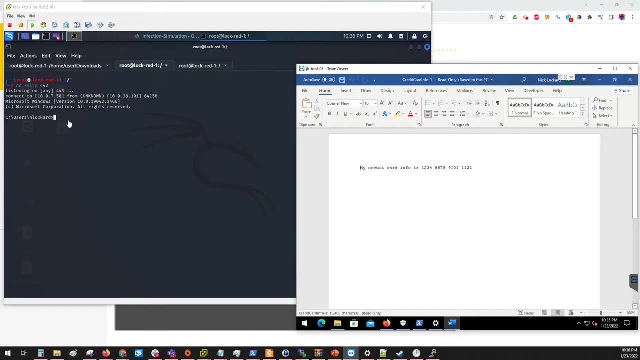 here, which, in this case, is a Word document. Now the victim computer here is running Office 2021,, as seen here, also fully updated and patched, And on the left hand side here, if you keep an eye on it, you're going to see what's going to happen As this Office document opens up. now stuff, just 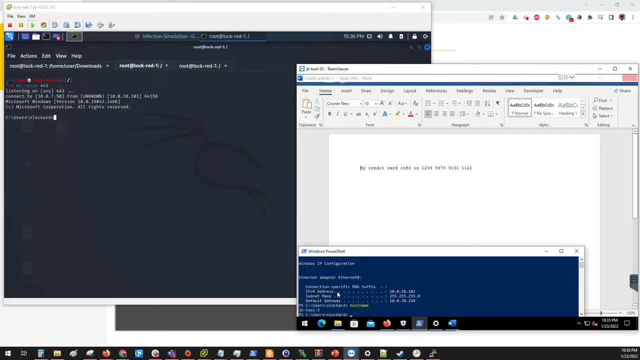 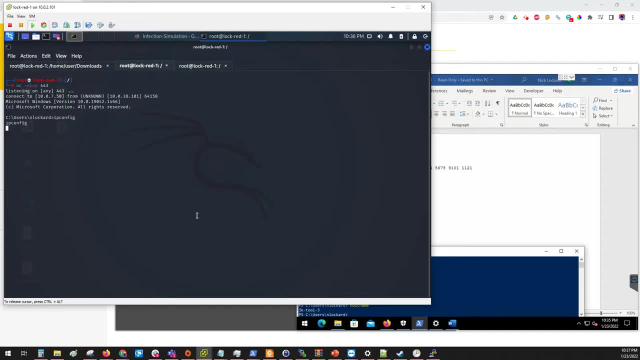 started happening on the left hand side here And you can see down in the bottom left corner here. this is the IP address of the victim And if the attacker runs the command ipconfig, you can see that they are seeing the exact same IP address and host name of the system. 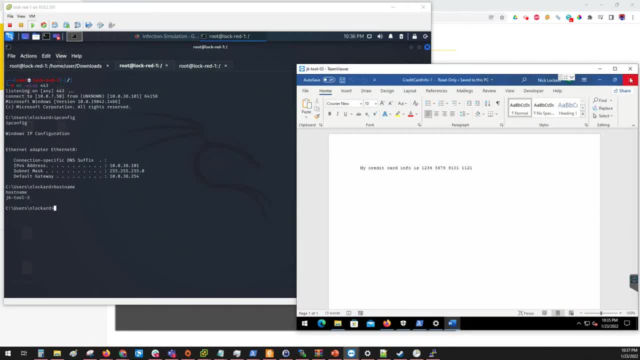 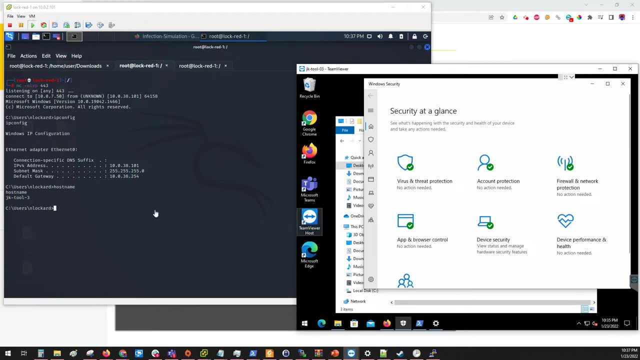 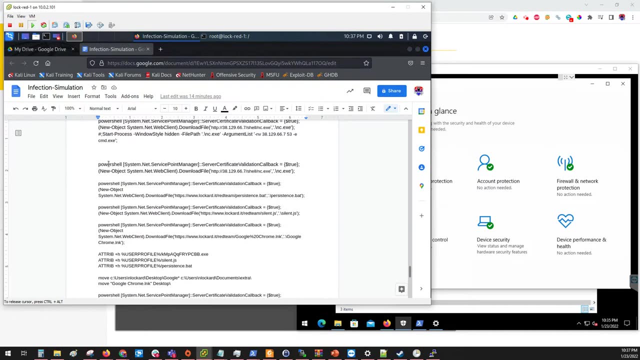 So the attacker has successfully gained access to this computer through a Word document, and there were no alerts, no detections whatsoever. That's how easy it is. Now the next steps that the hacker will need to do is to be able to maintain access. We call this persistence. And then they also need to. 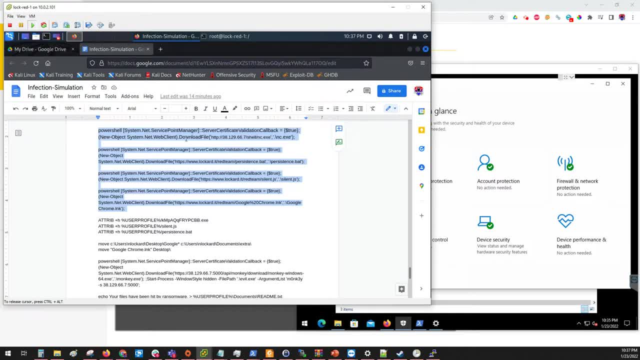 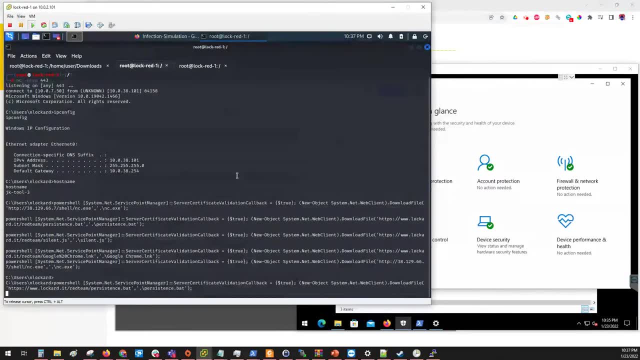 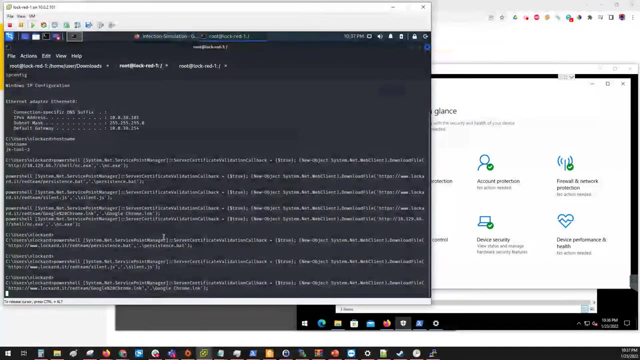 get their ransomware on the computer. So the hacker has written up some commands here that they're going to go ahead and paste in to the command prompt here that they've got access to, And this is downloading all of these different files And once these files finish downloading, this is going to allow the attacker to maintain. 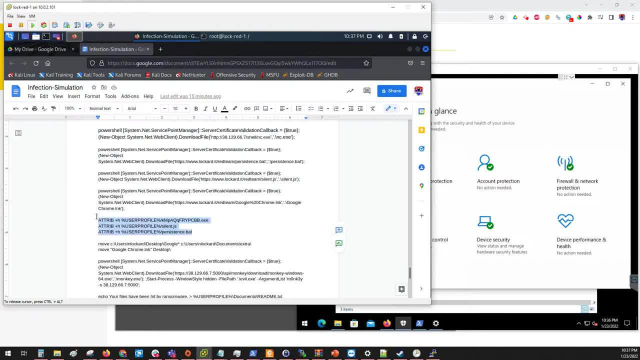 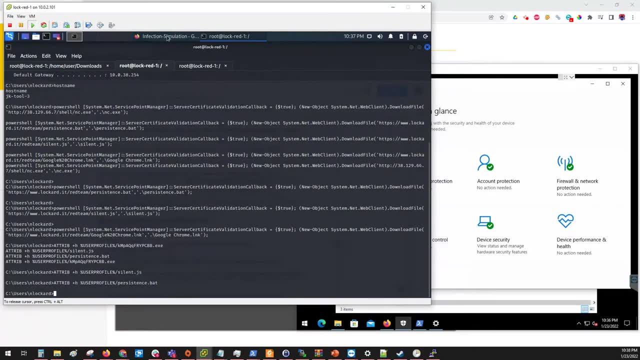 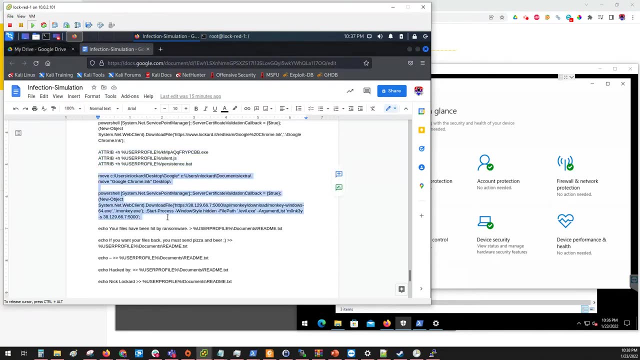 their access by every time, even if the computer gets restarted. In this case, what they're doing is they're backdooring to Google Chrome, And now they just made the executable and all of the things they just downloaded hidden, So it's much harder from a forensic perspective to be able to find it. 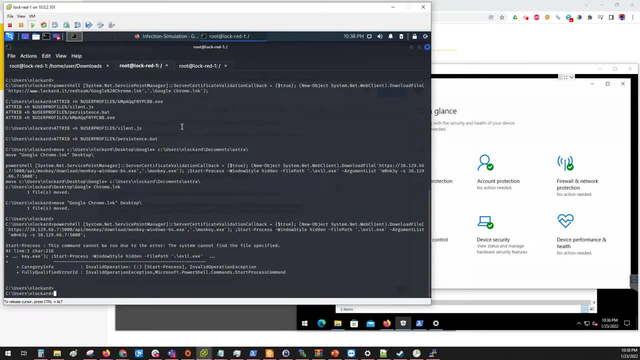 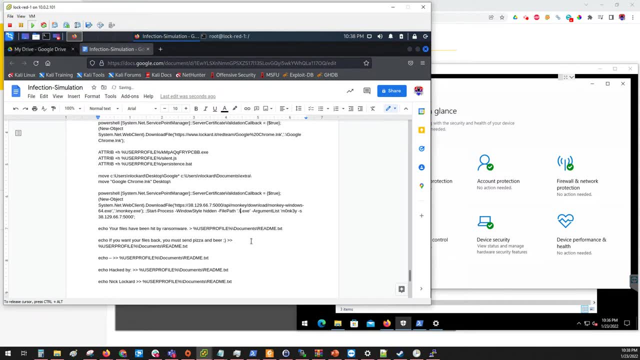 And now they are starting to download the malware. All right, Now, at this point it looks like actually there was a mistype here. Let me go ahead and correct the spelling here. It is now called this: Let's try that one more time. 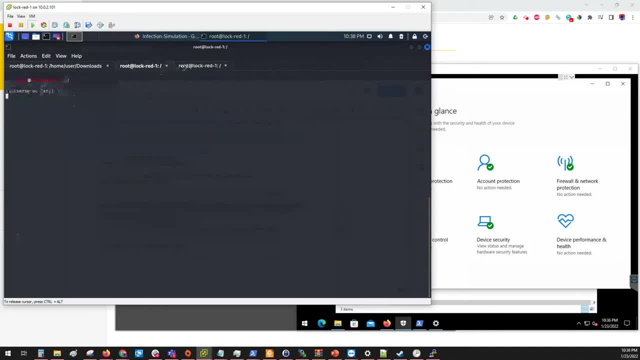 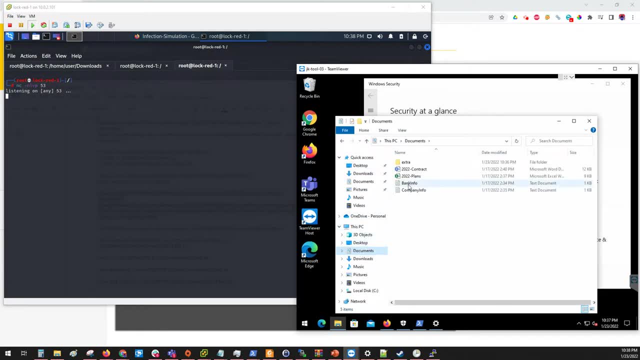 There it goes. All right, That's running now. So now what I wanted to show is how the persistent connection works and also what the attacker can have access to. So in this case, in the documents you can see- there's some documents here. There's a file called bank account number with a bank. 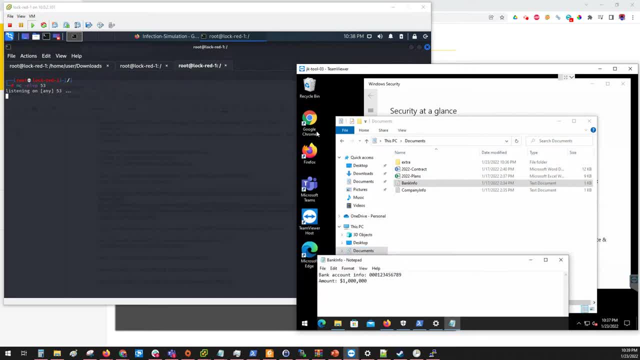 account amount. Keep that in mind, because what we're going to do here is we're going to just double click Google Chrome to simulate the other backdoor firing off And, as you see it did, It's coming over a different connection, And then you're going to see Google Chrome will open up. 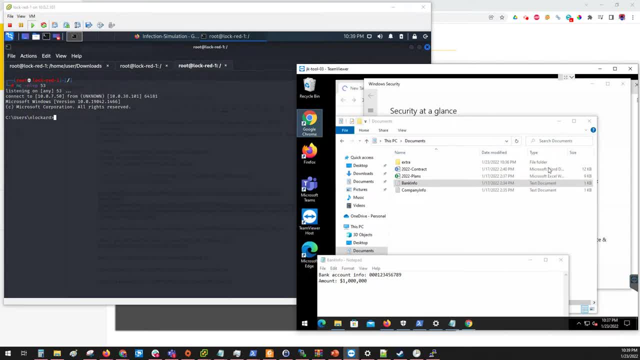 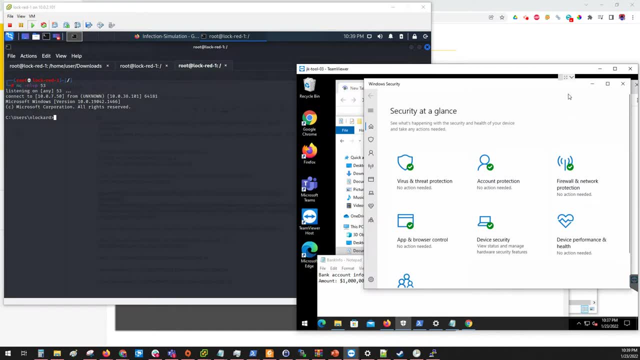 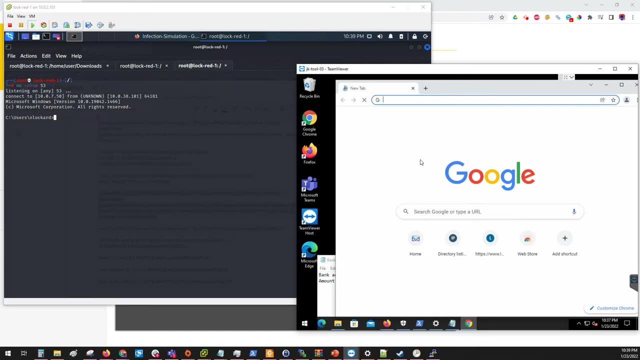 normal. So no pop-ups, no warnings, nothing at all. that would give an indication that there was a problem. As you can see, Security Center still says all is well And we'll go ahead and minimize this And we'll go back here to Google Chrome And it's Google Chrome. So if we do a Google search on 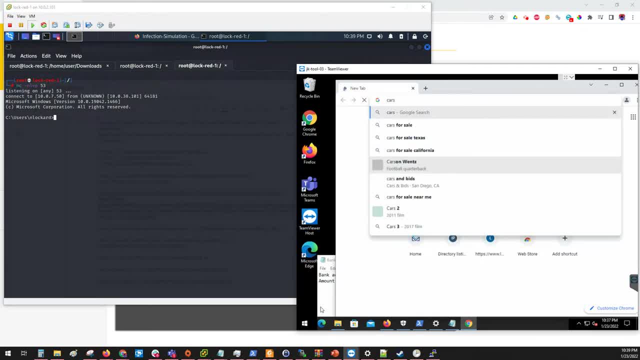 let's say cars. everything is running as intended. Now, this is a little bit slower system. one reason why it's running a little slow: It doesn't have many resources. It is a virtual machine, But, as you can see, it is Google Chrome. It is returning what you would expect to see if 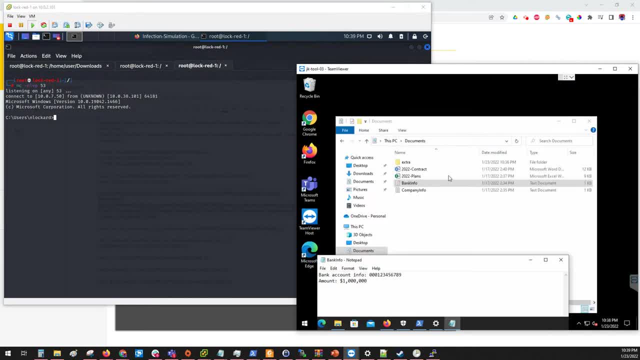 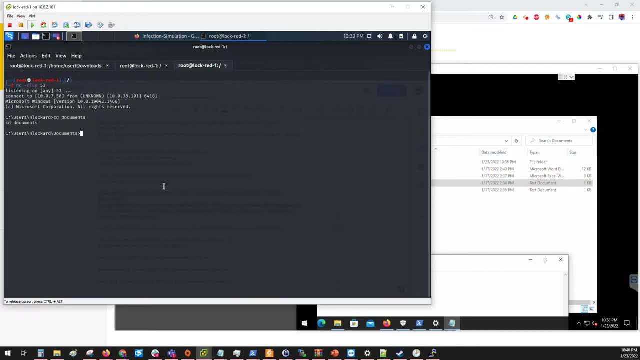 you did a Google search on that, And if you close out Google Chrome, we still have the connection. Now, what I wanted to show you was, if we go into, let's change the directory into the documents, we can see everything that's in the documents here And the attacker can simply do something. 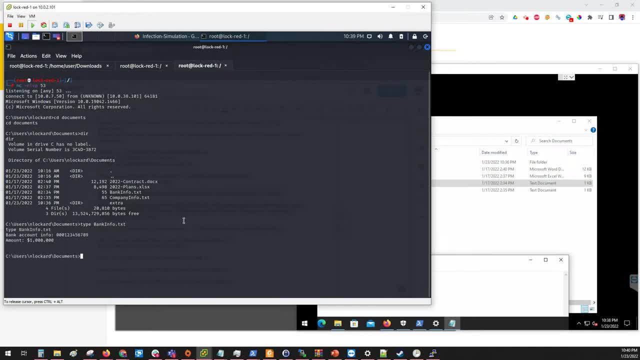 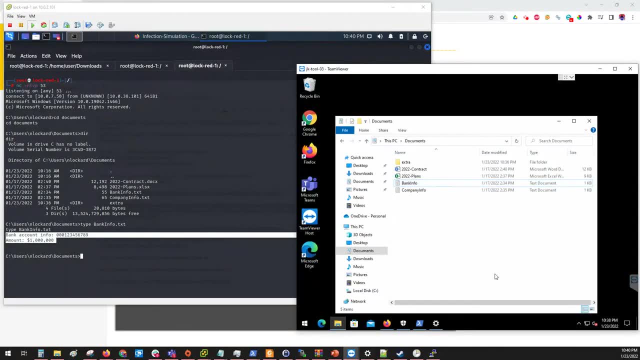 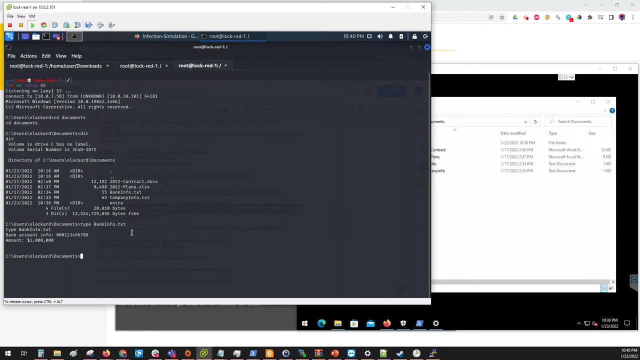 like this, And now they can read all the contents in the document as well. So, and the victim is no wiser that something has happened, that there's something on the system or someone on the system watching. So at this point we've got the ransomware started. It is running. 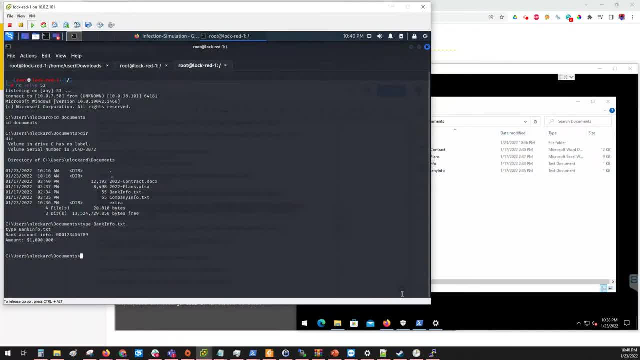 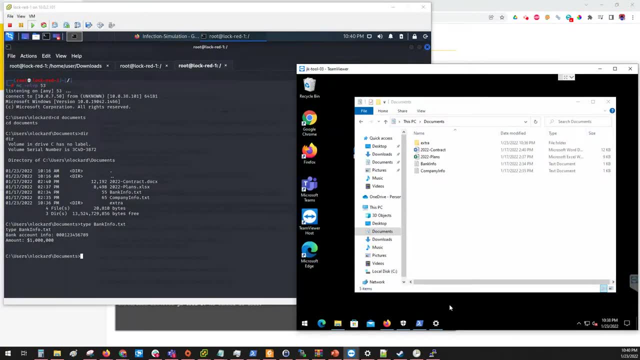 in the background, The ransomware is going to be doing a few things. It's going to be grabbing username and passwords out of memory, scraping a process called LSAS. It's going to start port scanning. It's going to look for other systems on the network. It's going 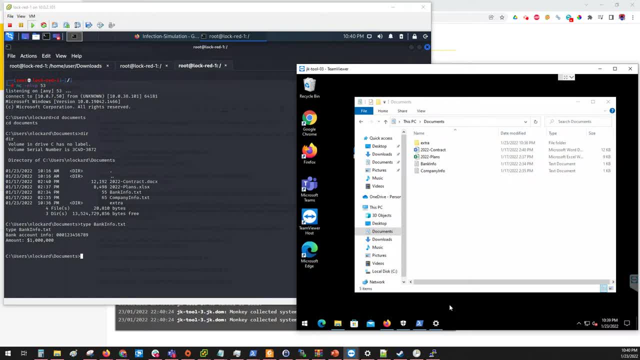 to look for systems on other networks And then it's going to try to do some lateral movement by connecting into those other systems using the credentials that it was able to get from this system. This system is joined to a domain, So this does simulate a business. 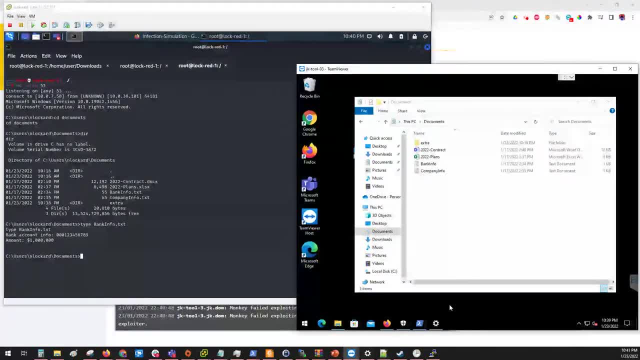 computer in a business environment with multiple systems And there are some exploits that it's going to try as well. They are safe exploits, meaning it's not going to fire something off that could potentially crash the system or lock it up or hang it up. in this particular case. Now we could do that, But in this example we're going to 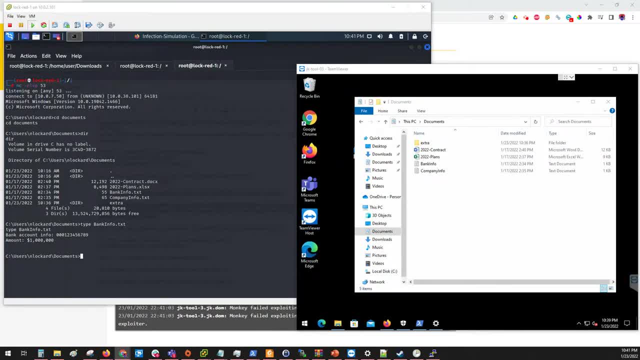 do safe exploits and see if the system's vulnerable to any of those. And since it's fully patched and updated, it's not going to find any vulnerabilities to exploit, But it is going to be able to scrape memory And then it's going to try to do some lateral movement by connecting into 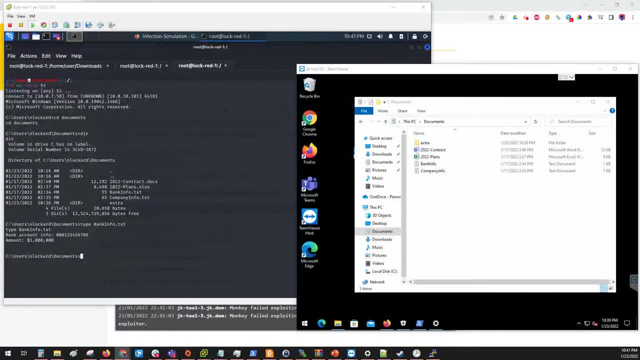 the memory and grab credentials that way. So this Ransomware will also then, most importantly, encrypt all the files in the documents that I've specified, And you'll see what that looks like. And so at this point, the attacker has full access to the system and the network, And I'm 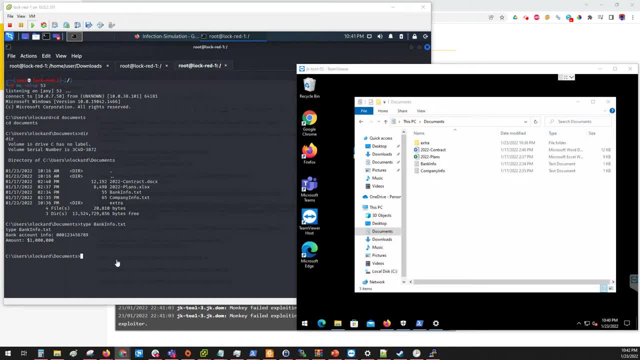 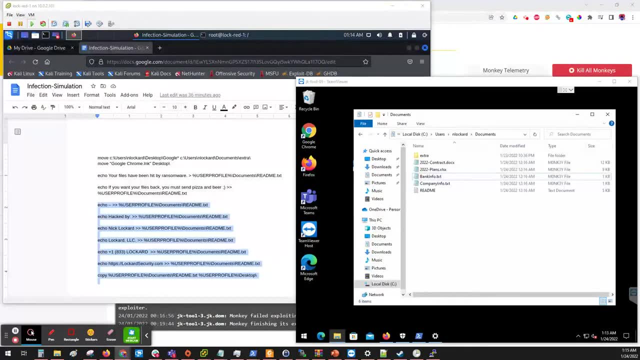 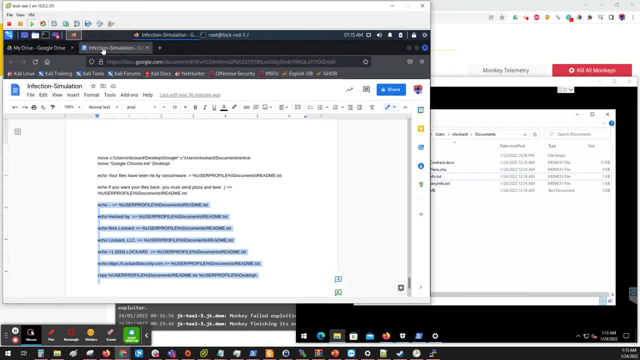 going to go ahead and pause it while we wait for the ransomware process to finish propagating to the network, And we'll pick it up right after it's finished. All right, We have completed all of the ransomware encryption. The last step is to build the actual ransom file. 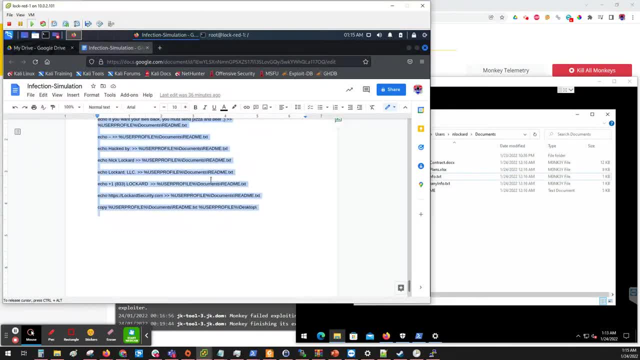 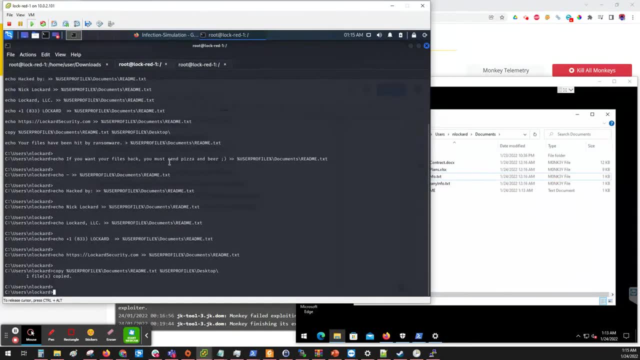 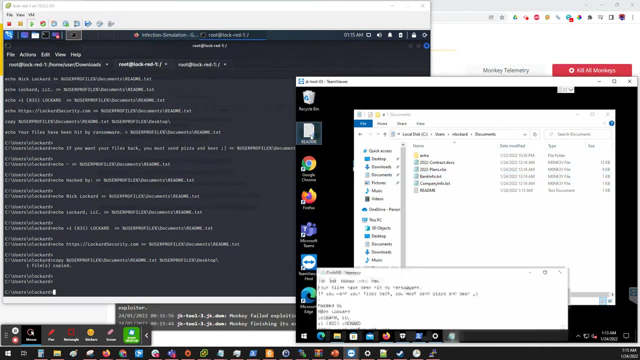 So we're going to go ahead and do that here. We're going to just echo in all of this text here like: so Perfect, All right. so now. the victim now sees a reading file on their desktop. If they open it up, here's what they see. 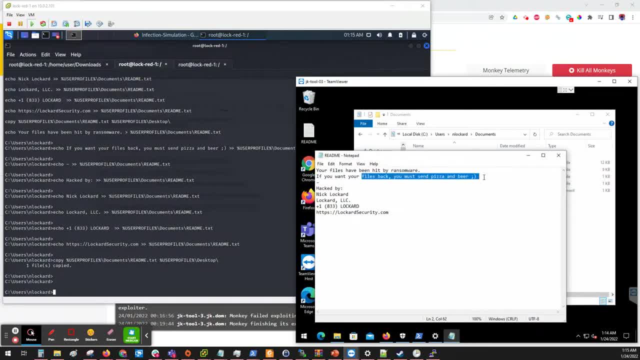 All your files have been ransomwared. Please send pizza and beer. Now the reality is, if this was a real life ransomware attack, this is where they'd be demanding Bitcoin. They would give you a link to figure out exactly how much it would cost. 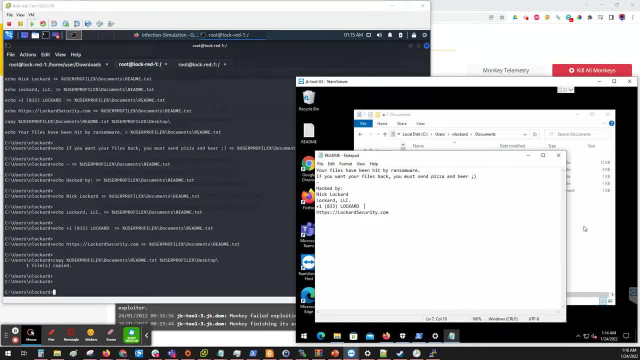 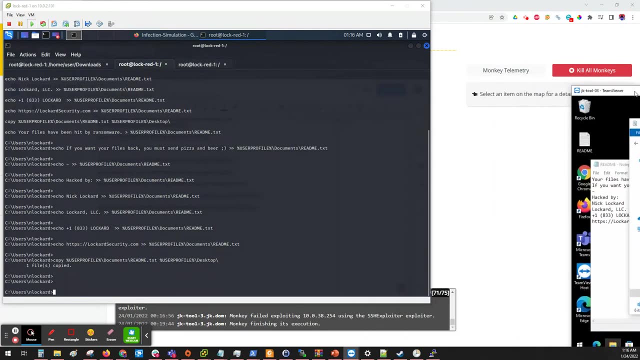 They send you to a chat room, basically, where you upload a file And at that point you'll get told how much and how to pay it. So I hope you all enjoyed this little demonstration. I would like to show a little bit more details. 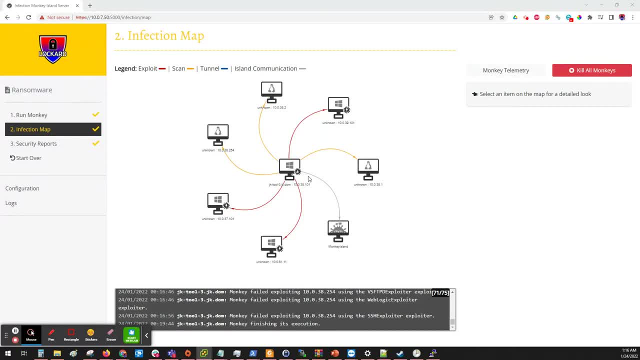 behind the scenes of what we are waiting to complete. So, going back here, you can see the center system here. This is the system that we started, with that we sent the document to, And the gray arrow going outbound here is to the attacker box. 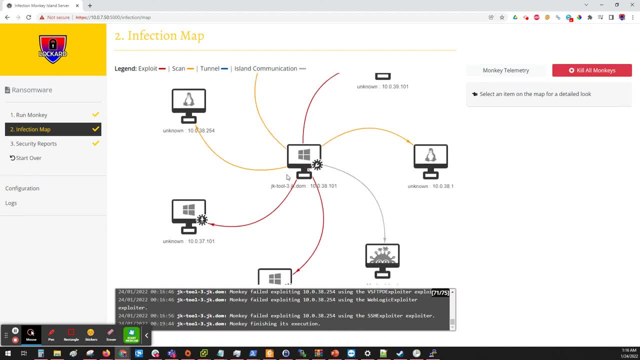 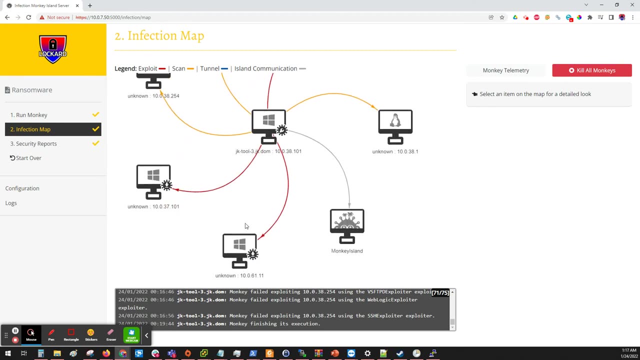 The red arrow. The red arrows are the systems that we were able to connect into by stealing the credentials of the one system and abusing that trust, and we were able to connect into others. You can see there's different IP addresses on these systems. 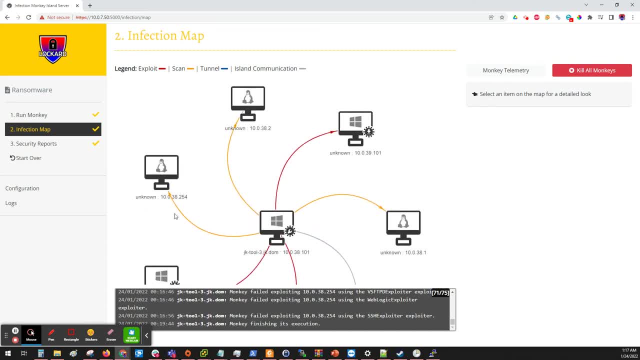 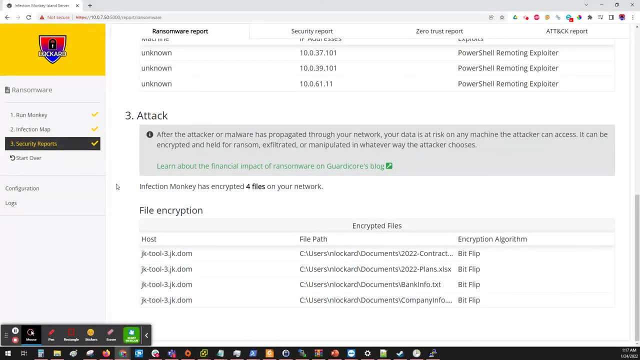 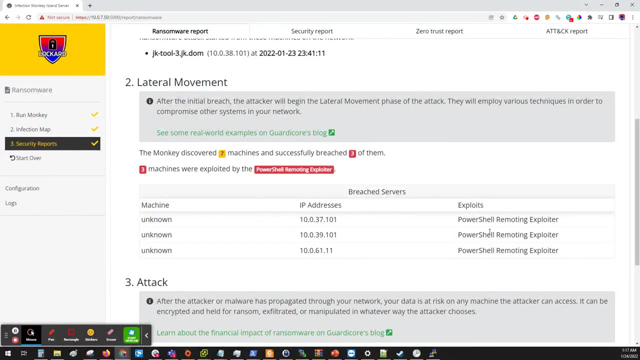 And then there were a couple others that we were able to identify by scanning, but we did not try to access them. The overall report shows a little bit more details. Please check the link below for more details. Thank you, and we can see. here are the files that were all encrypted. um. here are the different systems that 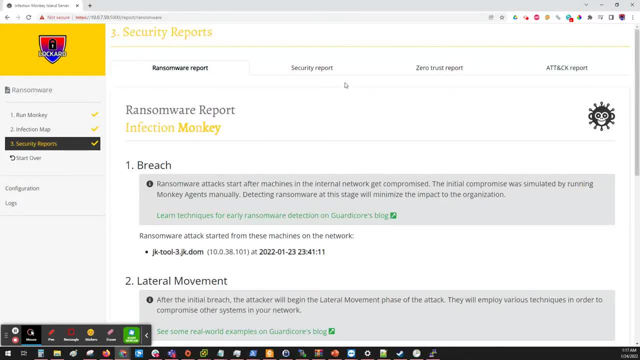 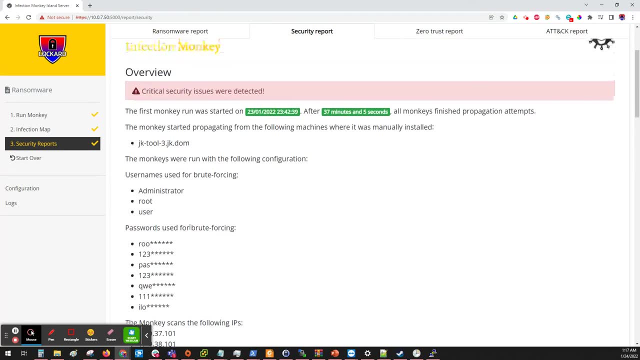 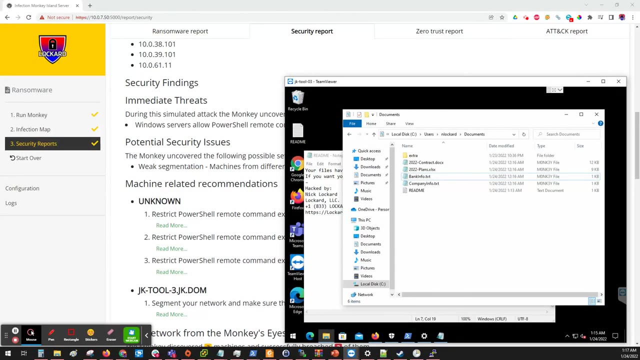 we were able to get access to. so i hope you all enjoyed, uh, everything here. we, um, we we did try a couple different type of attacks. not all of them did work, but you know, at this point, as you can see, you cannot rely solely on a single defensive mechanism. 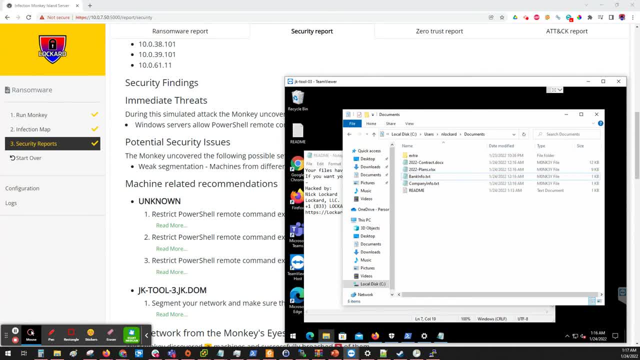 um, you know, such as antivirus or just a firewall, and so lockard security specializes in cyber security, both defensive and offensive solutions. it's one thing to have security in place, it's another to make sure that it's actually working as expected, and that's where we come in.